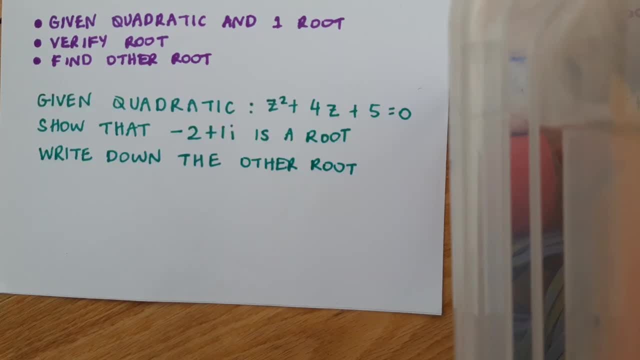 a couple of different ways in which we can do this. So my example is going to involve the quadratic z squared plus 4z plus 5 equals 0, and I want to show that minus 2 plus 1i is a root, and I want to 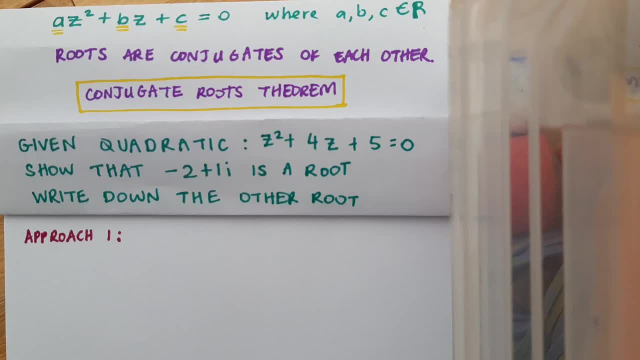 write down the other root. So approach number one is just the approach that we've used previously when trying to find the roots of quadratics. it's just to use the minus b formula. so minus b, plus or minus the square root of b, squared minus 4ac, all over 2a. Now, like I said, I've shown how to do. 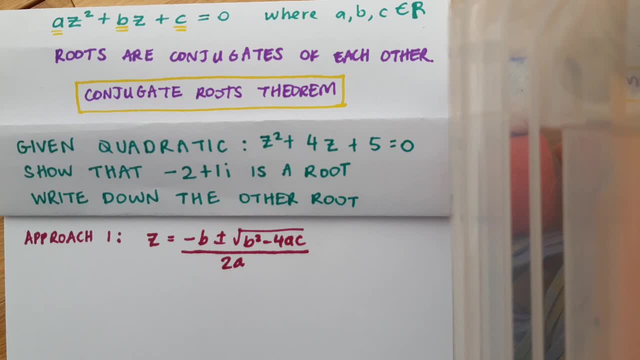 this in a previous video, so I'm not going to go through all of that again, but what I would like you to do yourself is to make a note. So if you have your a, b and c values for this quadratic, fill in the formula and see what you get. 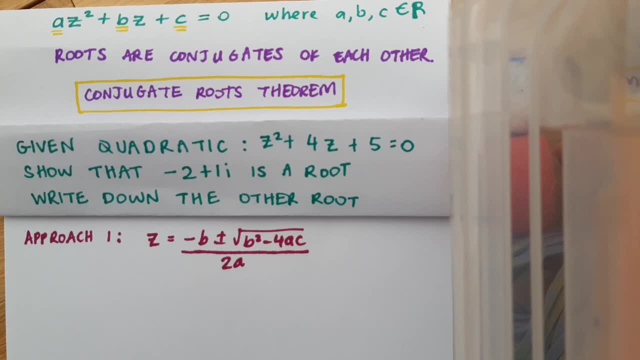 You're going to expect that minus 2 plus 1i is one of the roots and then, because of the conjugate roots theorem, I would expect the other root to be minus 2 minus 1i, and notice that this is the case because in this quadratic the coefficients and the constant are 1, 4 and 5, so they are all real. 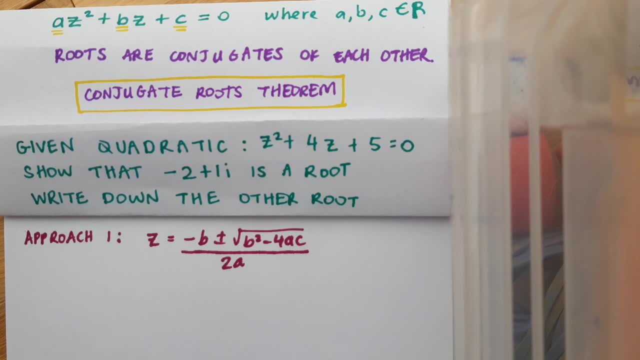 values. So take a moment, pause the video, work out the formula and see what you get. So take a moment, pause the video, work out your solutions to the minus b formula and see if you get them correct. and, following this approach, you can find fact. it's how you find, in fact, that z is equal to minus 2 plus 1i and the other root is minus 2 minus 1i, and that's what we expect it to happen. 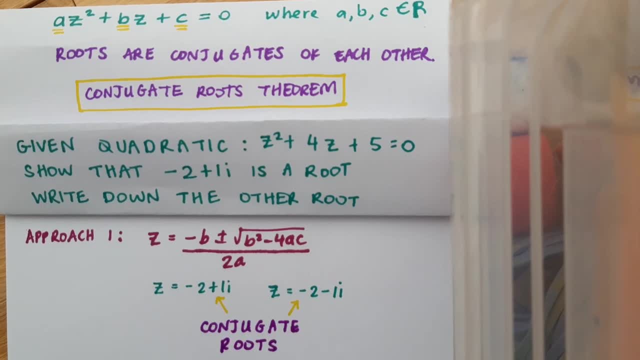 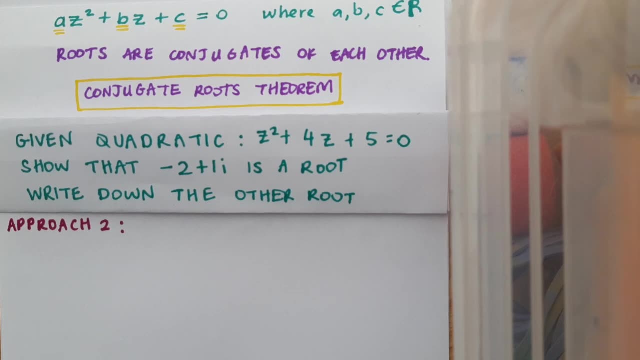 You can see that these two roots are conjugates of one another. Approach number two is an approach that we're familiar with from previously in algebra. If I want to confirm that some roots are conjugates of one another, I'm going to have to do this. 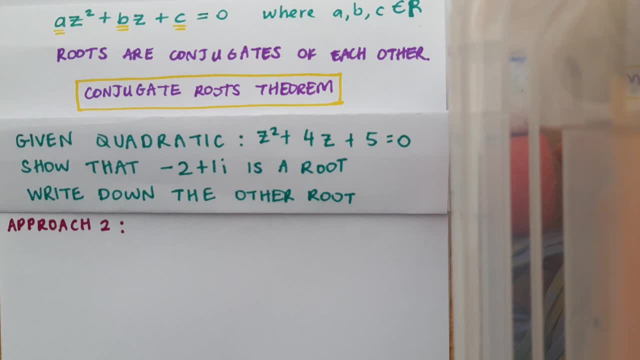 So if I want to confirm that some roots are conjugates of one another, I'm going to have to do this. So if I want to confirm that something is in fact the root of a function, well then all I need to do is sub it in, and I should expect for the result to be equal to zero. 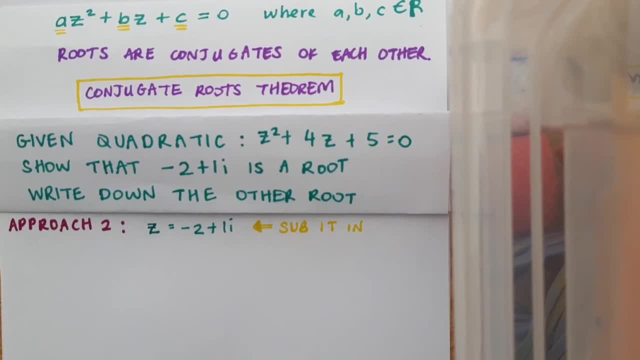 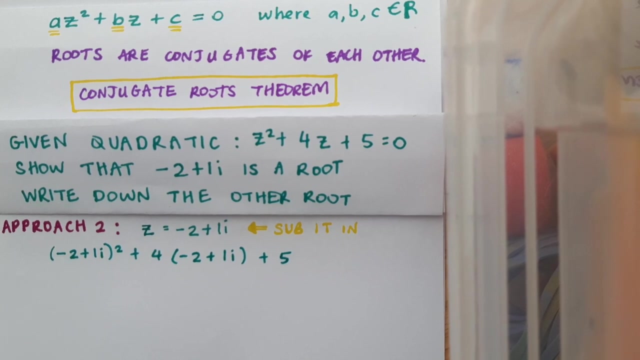 So let's take z equals minus 2 plus 1i and sub it in for z that we see in the quadratic and again pause the video here. do that yourself and see if it does in fact come out as zero that we expect. So I've replaced z with minus 2 plus 1i. 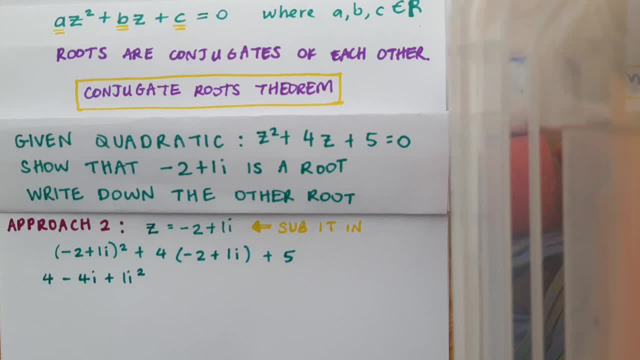 I'm squaring out my first bracket. just be careful with that. and multiply out my second bracket and stick the plus 5 at the end. Now just a little bit of tidying up. So of course I see an i squared there and I know to replace that with a minus 1. 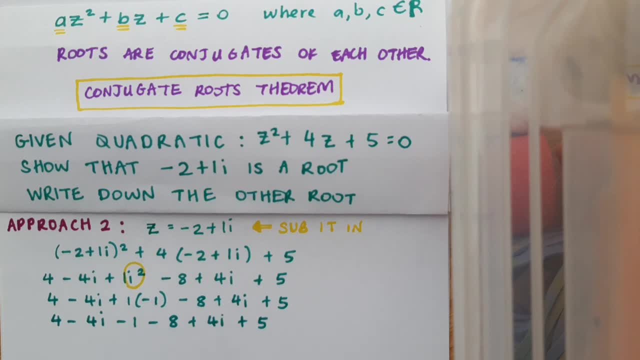 and on inspection that I can see that my real terms and I put them together, 4 minus 1 is 3 minus 8 is minus 5 plus 5 is 0. So these all effectively cancel out and minus 4i plus 4i is also zero. 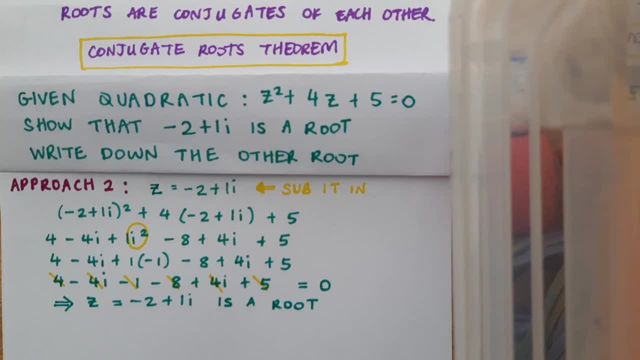 So this confirms that z is in fact a root. Now that I'm sure that minus 2 plus 1i is a root, I have direct access to the second root, and that is, of course, because the quadratic that I'm dealing with, z squared plus 4, z plus 5 equals to zero- has real coefficients. 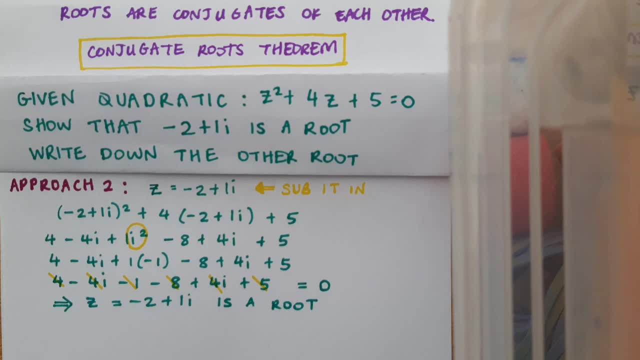 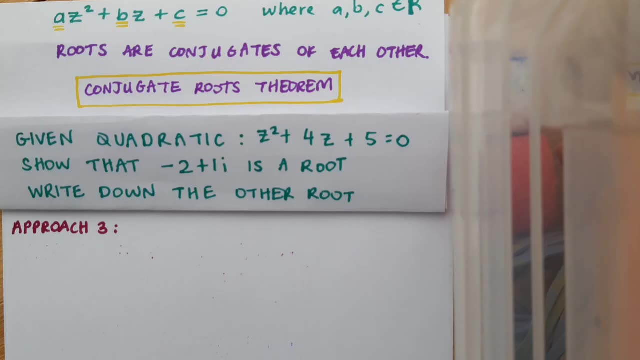 So that means that once I know one of the roots, the other root must be the conjugate of that root. So in approach 2 we relied on the roots to figure out the solution. In approach 3 we're going to look at how roots and factors are related and use factors to work towards our solution. 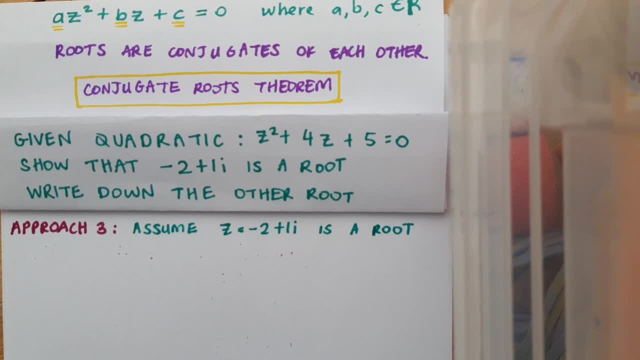 So I'm going to start by assuming that z equals minus 2 plus 1i is in fact a root, and if that's the case, then the other root, of course, would have to be a root. It doesn't have to be its conjugate, because of the nature of the quadratic with its real coefficients. 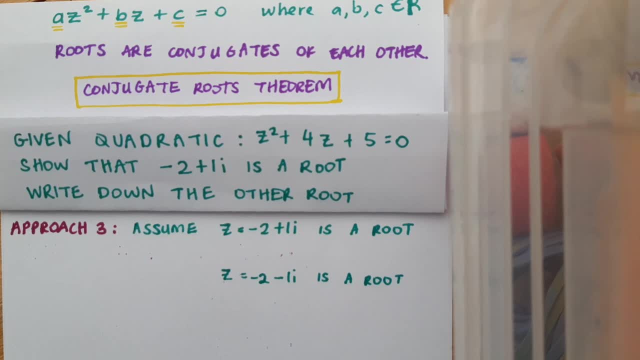 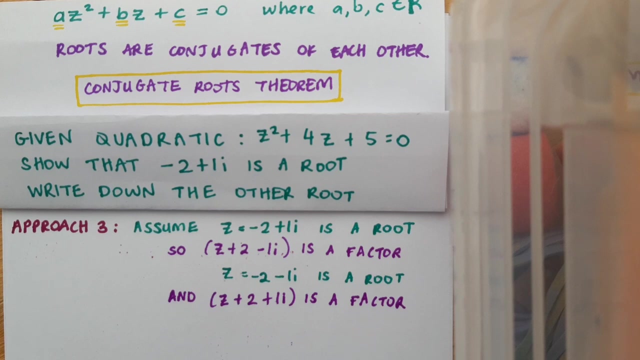 And I'm then going to say: well, if these are the roots, I can figure out the factors of the quadratic. And of course I simply do that by bringing this information on the right hand side of the root equation over to the left. So if this is the case, then I've got two factors: z plus 2 minus 1i. 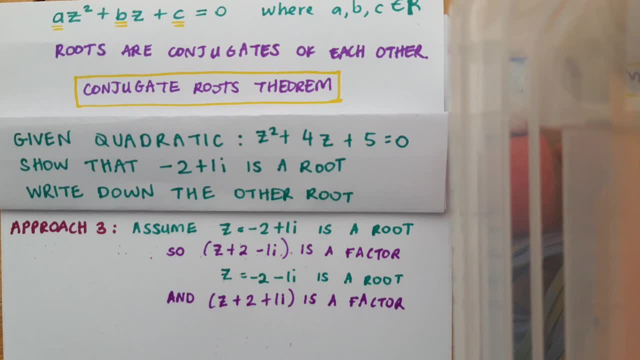 And z plus 2 plus 1i, And of course I'd expect, when I multiply the factors of my quadratic together, that I would get the quadratic in question. So I'm going to do that and see what happens. Now I find that when multiplying this out, because you've got three terms in each bracket- it gets a little bit clunky. 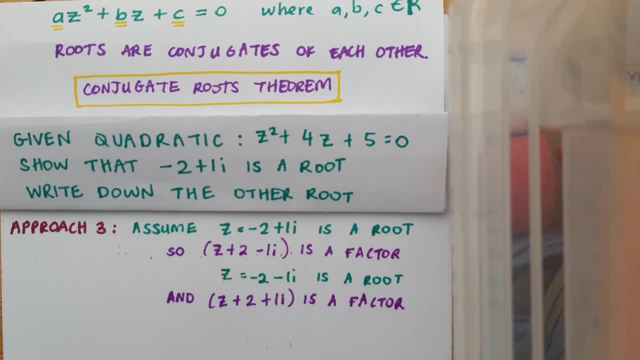 So I actually really like to represent this using the array, and you'll see why in a moment. Just to say, if you're not familiar with the array or you don't like it, it's totally fine to multiply it as normal, But I'm going to use the array. 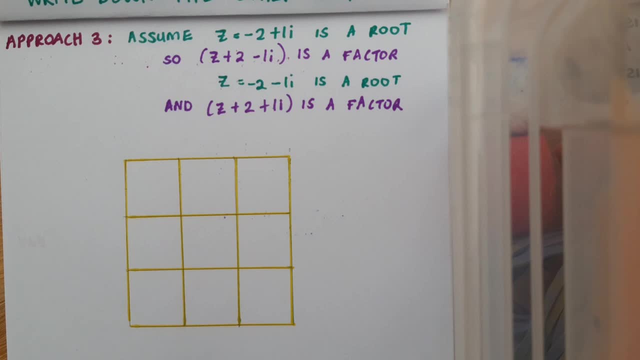 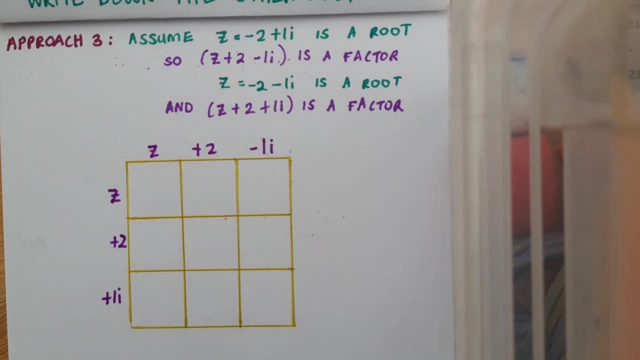 So here's my array. If I'm correct, I'm expecting that when I multiply out I should end up with that original quadratic, z squared plus 4, z plus 5.. So I'm putting my terms from my brackets along each of the sides of the array and I'm going to multiply into it. 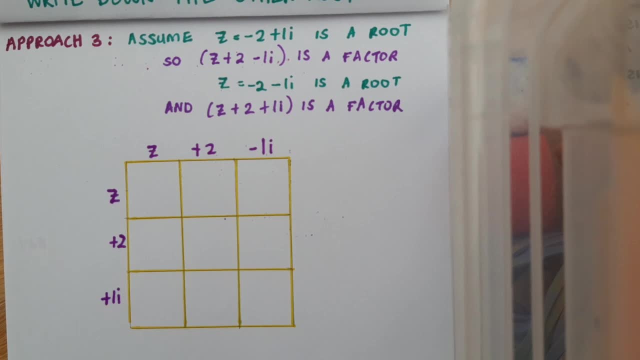 At this point, pause the video, multiply it out yourself and see what you get. And see, do you notice any nice kind of symmetries going on as you work through this multiplication? So here's my first row and my second row and my third row and just a couple of observations here now. 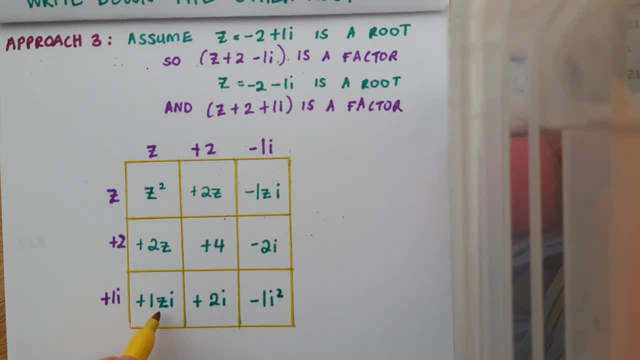 You'll see that, looking at this box here, the plus 1zi. on the other side I've got minus 1zi And they're going to cancel out. I've got plus 2i and minus 2i And they're going to cancel out. 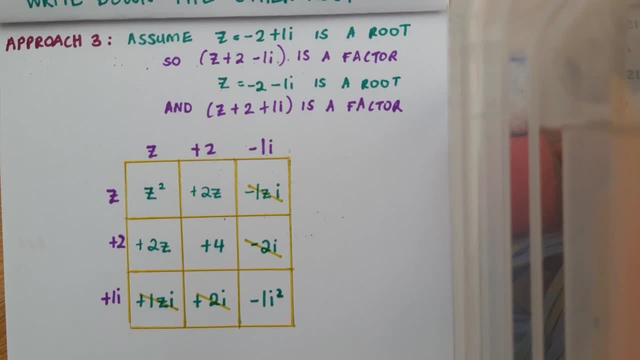 I've got minus 1zI got the i squared in the corner and i'm going to have to replace that with minus one and just note this little cancelling pattern that occurs. that's always going to happen if you have created your factors from conjugate roots. so it's nice. it kind of tidies itself up in a way. you're also going to 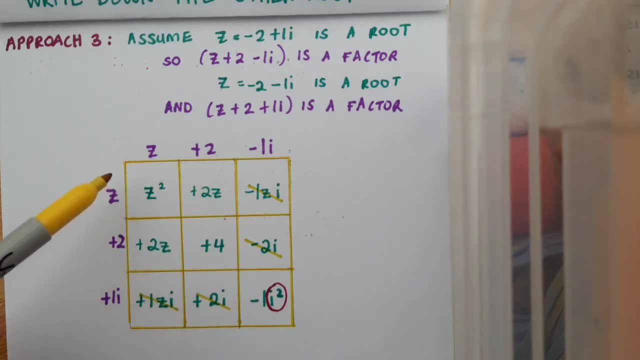 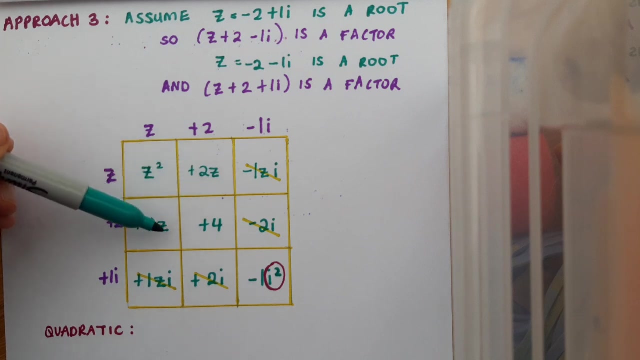 find that this information here is going to be a perfect square that obviously gets disrupted by this minus one. i squared in the corner, so nearly there. i'm just going to assemble it now. so my z squared is going to go first- my z terms are always going to be on this diagonal- and then i'm going to 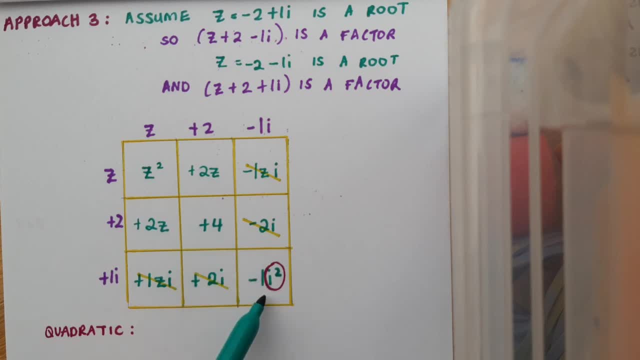 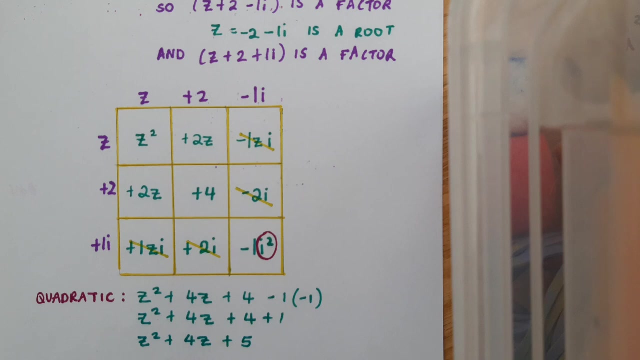 have my constant formed by this diagonal here. of course this doesn't look like it's real right now, but that minus one will go in and ensure that it actually is. and then, last little step, and i've arrived at my quadratic. now you might think this is slightly overkill, given the slightly short. 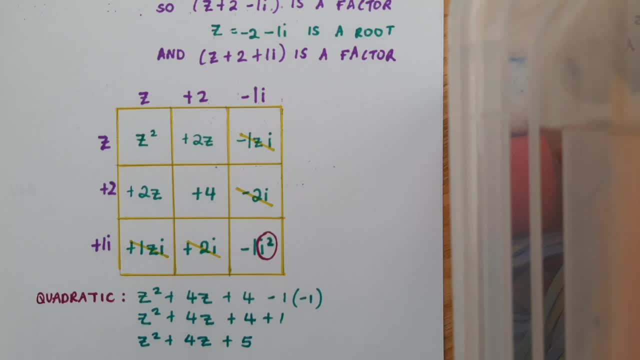 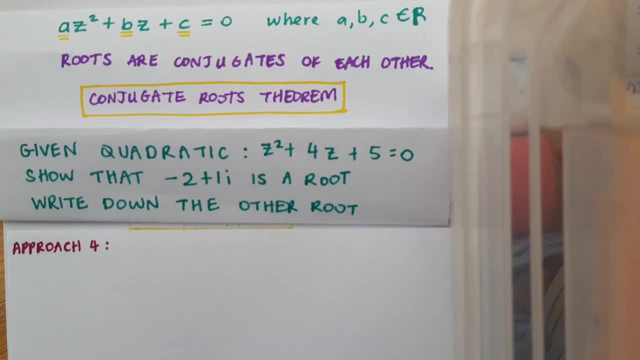 build the quadratic if it's unknown to you initially. and then, finally, i've got approach number four, and approach number four we're again familiar with from previous algebra chapters. so there is a formula that you can use to create a quadratic if you know what its roots are. 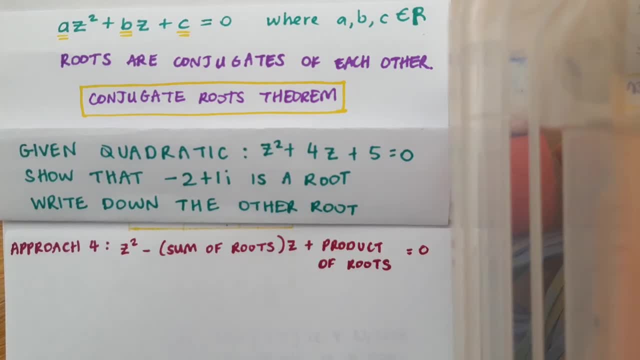 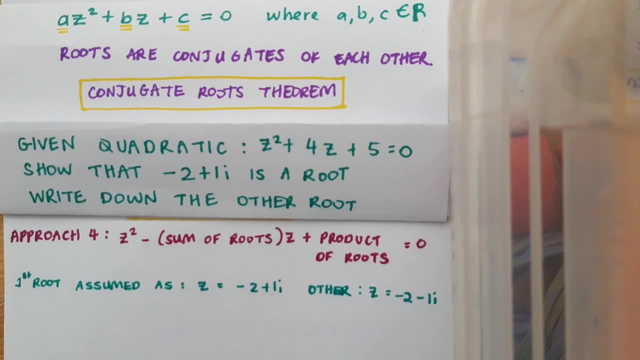 and that formula is z squared minus the sum of the roots, times z plus the product of the roots. so again, i'm going to start this case by assuming that the root that i'm being given is correct, in which case my other root would have to be its conjugate. i'm going to build the quadratic. 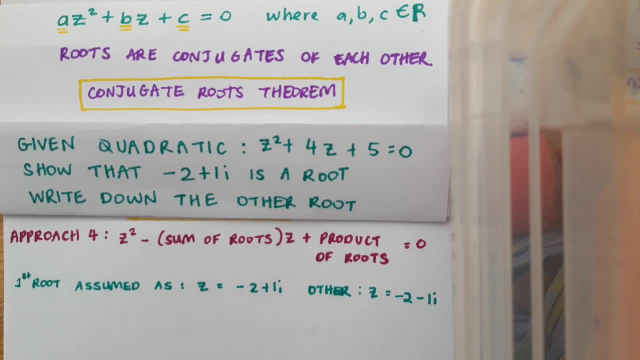 if i get z squared plus four- z plus five equals zero- then i'm satisfied that minus two plus one, i is a root, and of course then i also have my other root, which is the conjugate. so it's simply a question of subbing in in this case. 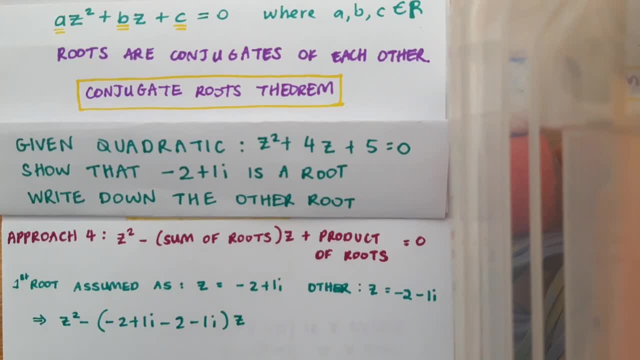 so i first of all fill in the sum of the roots. now notice: some means that i'm adding the roots together and you might say to yourself: well, why is it a minus here? but i'm adding minus two, so plus, minus is a minus. and i'm adding minus one, so that's going to be a plus by a minus is a minus. 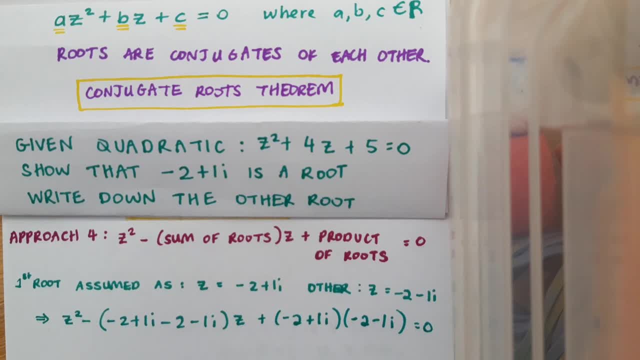 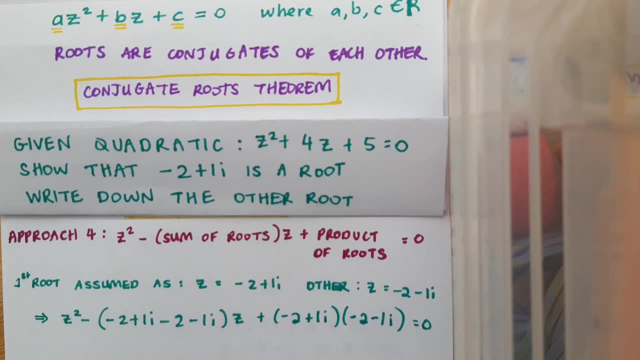 as well. hence the negatives here. so a quadratic with these two particular roots would look like this, and then it's simply a question of tidying it up and seeing: does it conform to expectations? ending up as z squared plus four, z plus five equals zero, and then i'm going to add minus two. 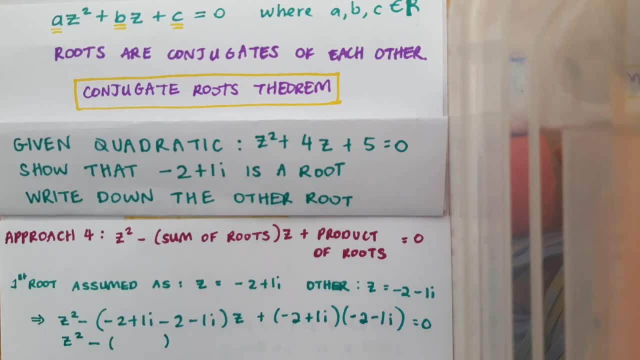 plus five. well, i can see in that first bracket that i've got plus one i and a minus one i, so they're going to hop off and i'm going to have minus four left inside the bracket with a z. and then when i multiply out the two brackets at the end, notice it's a difference of two squares if. 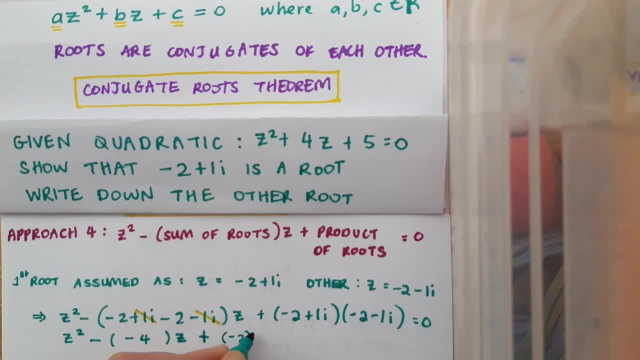 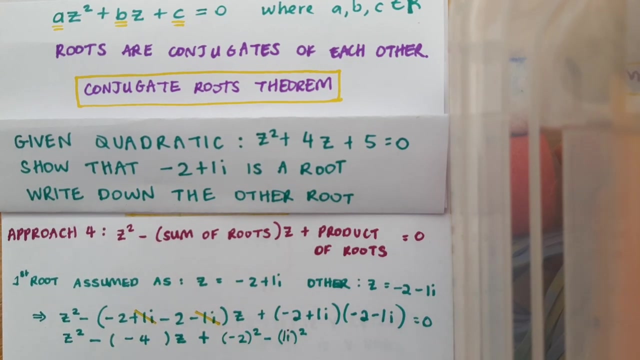 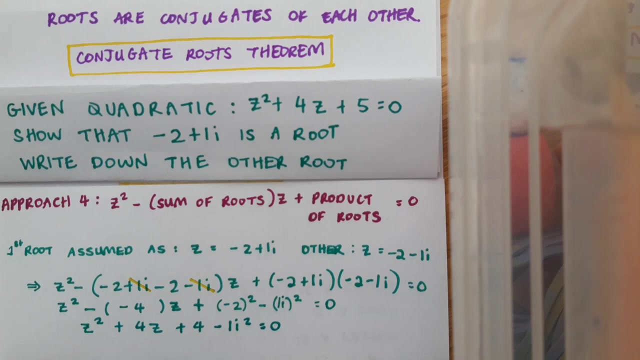 you like. so you can say it's minus two squared, minus one squared- sorry, of course, that should have an i in it, shouldn't it? so minus one i squared, and then it's simply going to be a matter of just multiplying that out, and i'm almost there.